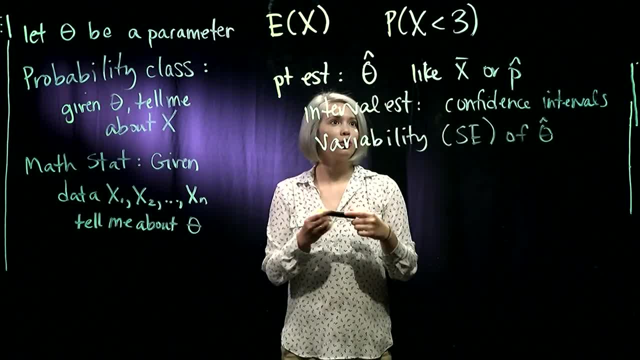 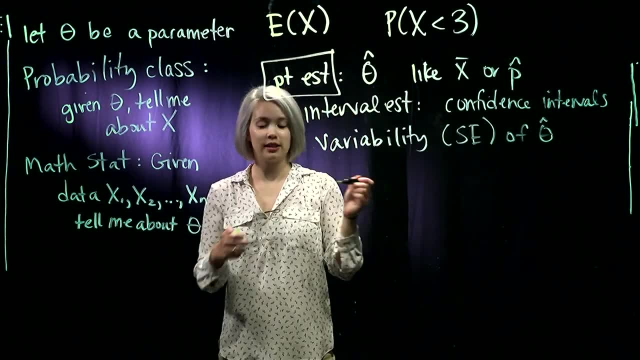 So usually we call that variability standard error. So those are some things that we could be looking for. So the first thing that we're going to be talking about in this class are point estimates. So point estimates are estimates. So point estimates are estimates. 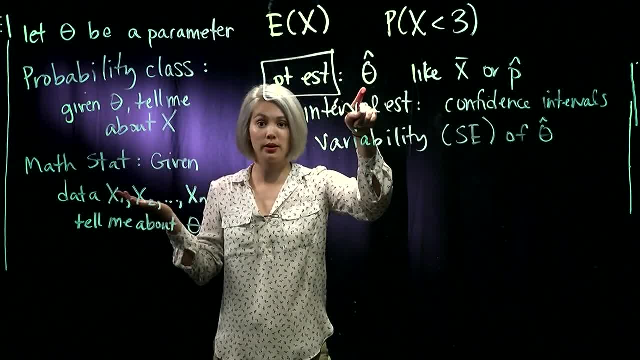 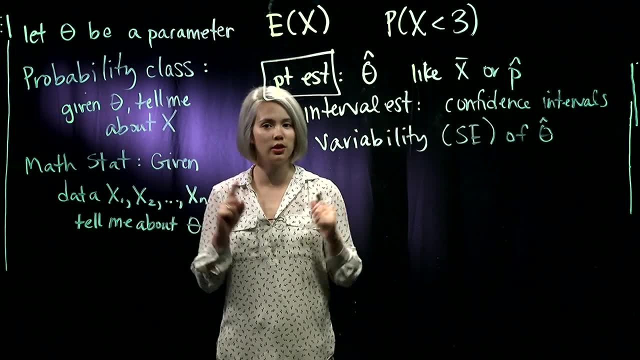 Of our parameter, theta. so usually we might denote those like theta hat. And since it's a point estimate, that means we're only guessing one single point. So we're not guessing an interval, just one single point. So we're trying to look for our one best guess of what theta might be. 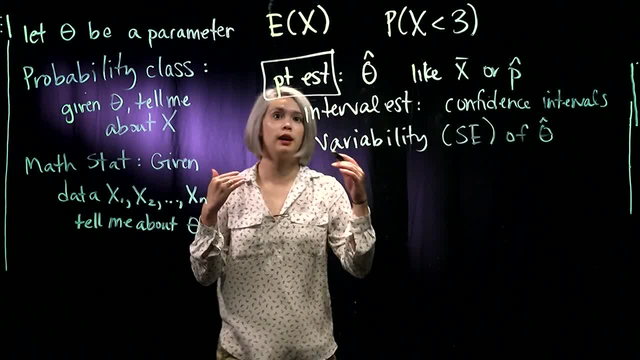 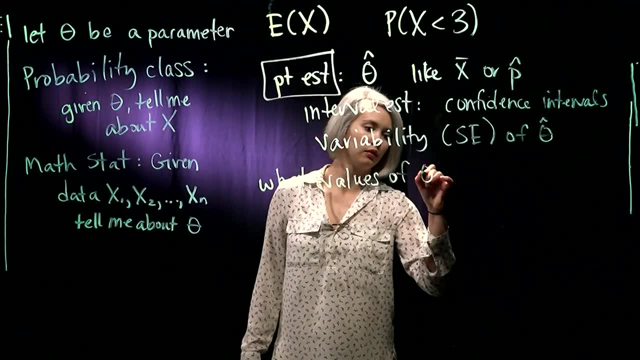 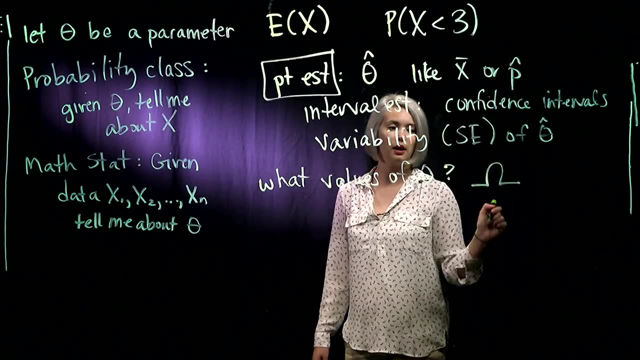 Some things that we should probably think about before actually beginning our point estimation is we need to know what values of theta are fair game. So what values can theta be fair game? So what values can theta take on? So we usually call this capital omega. 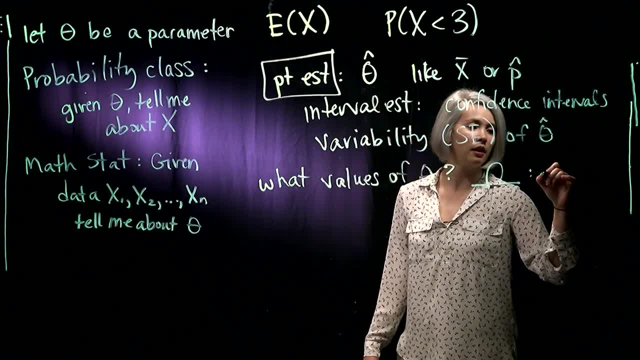 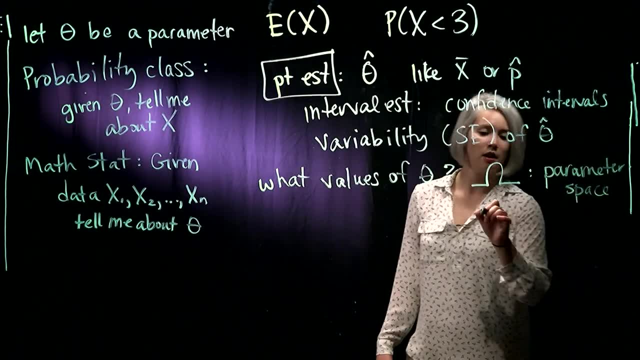 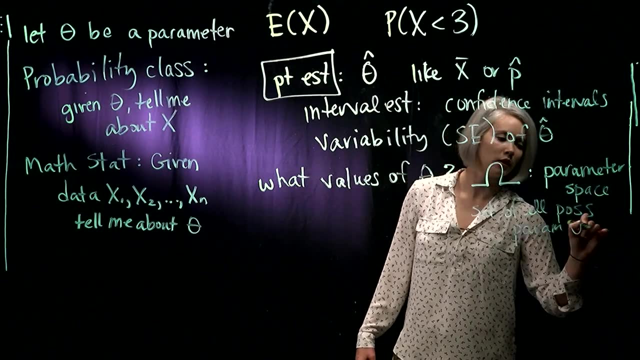 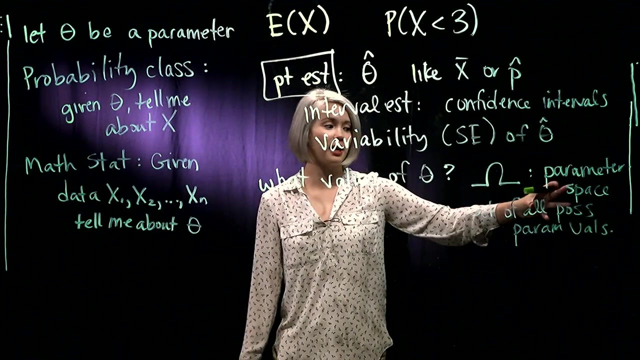 And so this is the parameter space. So this is the set of all possible parameter values. So this is important because we don't want to be guessing like negative numbers for variance or something like that. We want to know What are all the possible values that our parameter could take on. 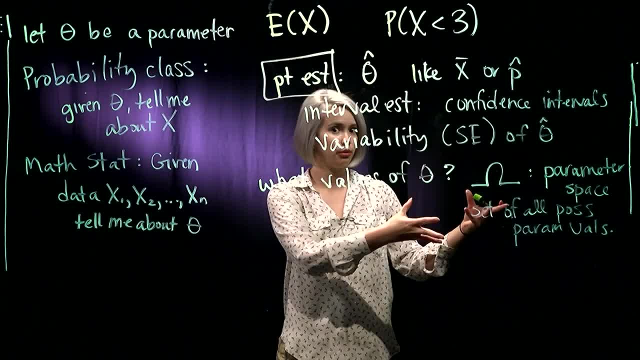 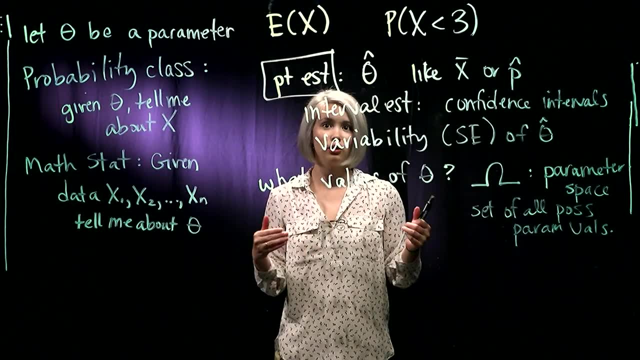 And then we're going to try to guess a point, get a point estimate that's in that parameter space. Another thing that's important to know before we get into point estimation is we need to see: is our point estimate on average going to be estimating our parameter? 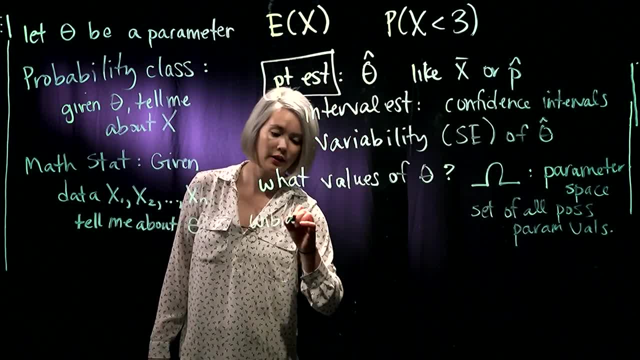 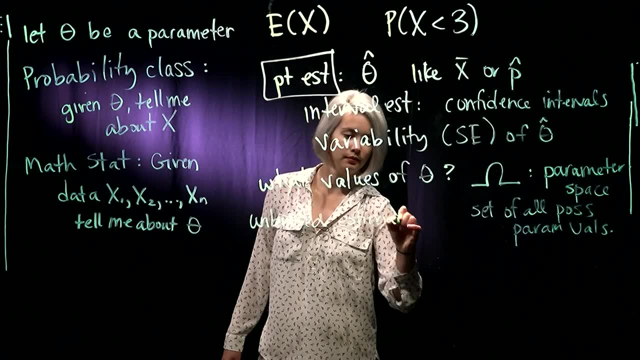 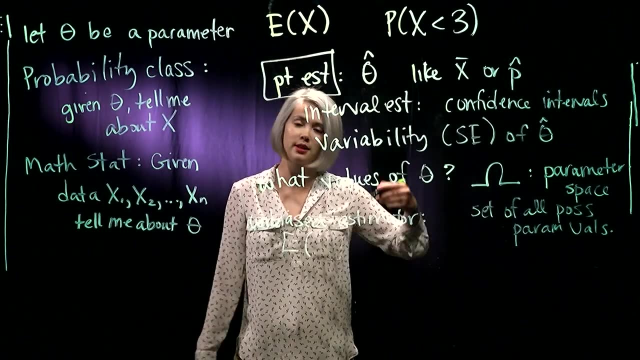 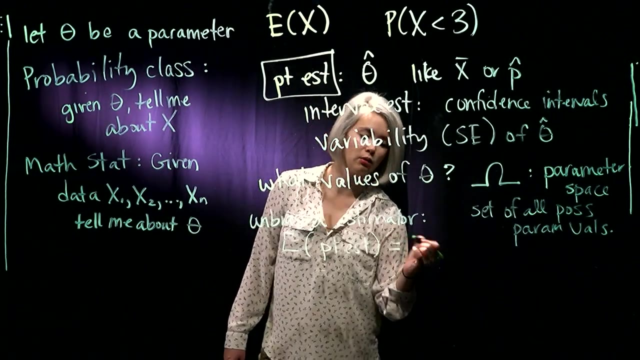 So we call this an unbiased estimator if it does on average estimate our parameter. So, in other words, we're talking about on average, So we're looking at the expectation, because that's our like, long run average of our point estimate. We want that to be equal to whatever parameter we're estimating. 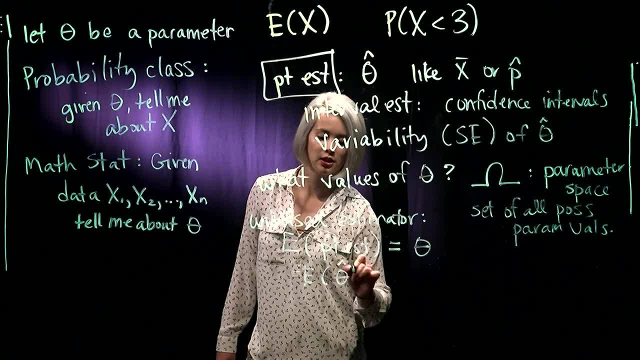 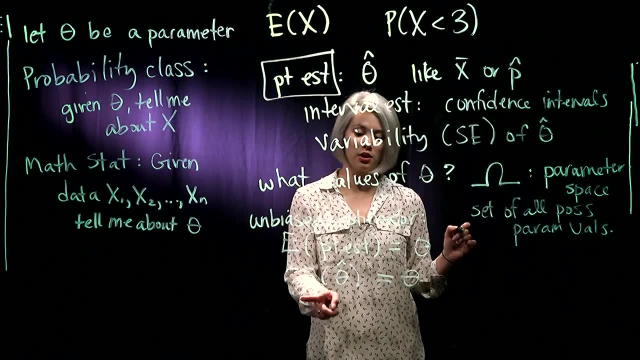 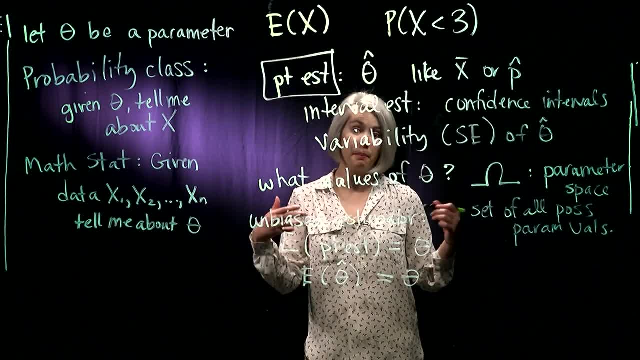 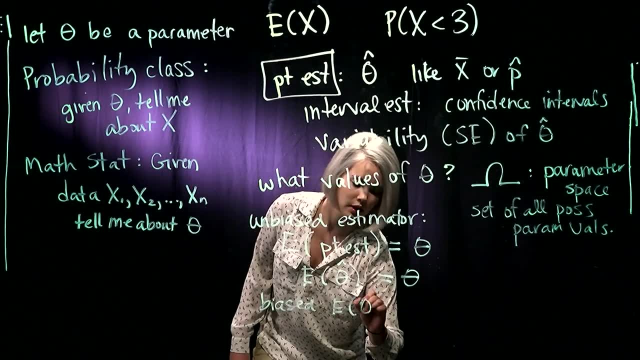 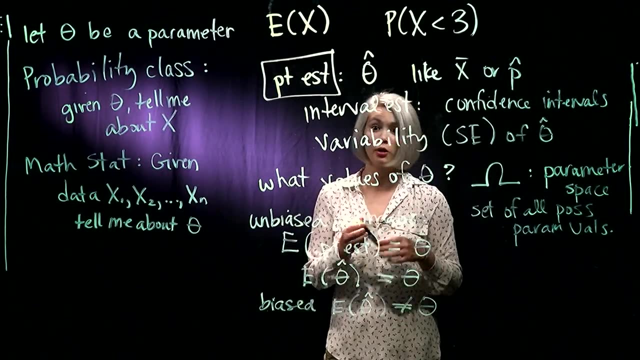 our point estimate is equal to our parameter, and if we have a biased estimator, then that means that the expectation of theta hat is not equal to theta. So that is, in a nutshell, some of the things that we're going to be talking about when we talk about point estimates. 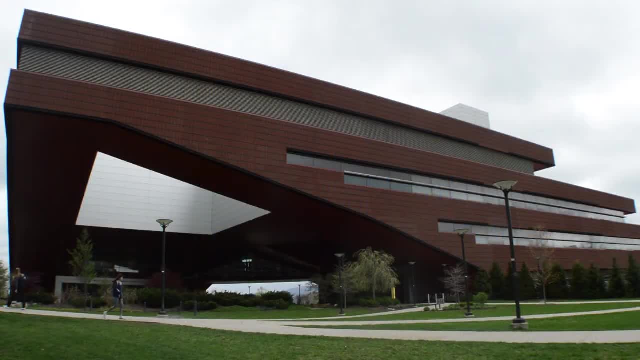 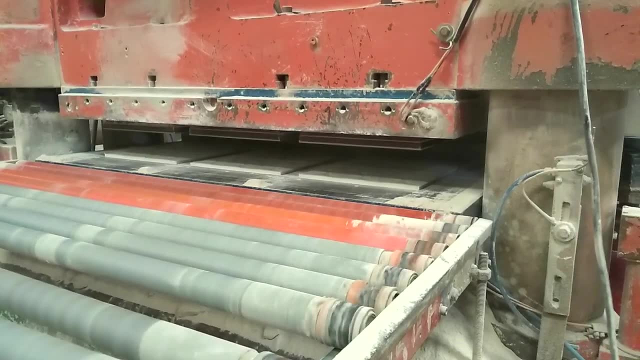 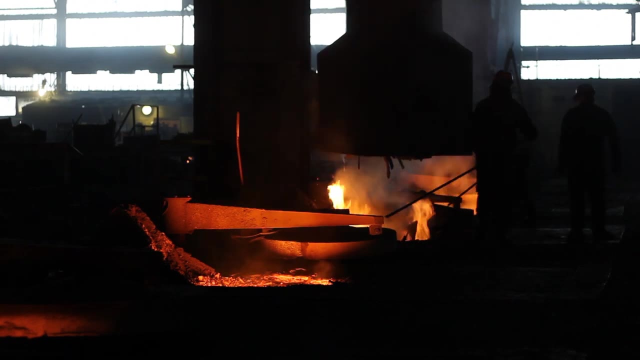 Penn State researchers recently discovered a way to revolutionize a widely used manufacturing process known as sintering. Sintering is the process of compacting and forming a solid mass by heat or pressure. This is traditionally done at temperatures of more than a thousand. 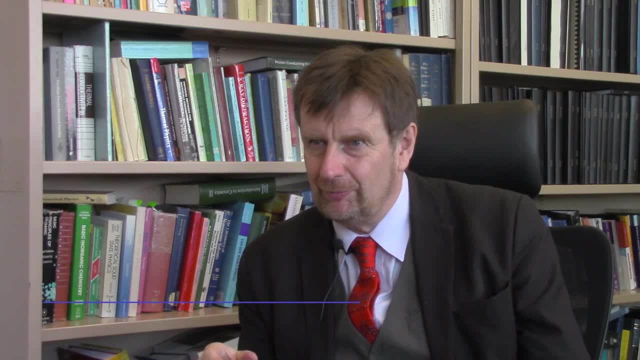 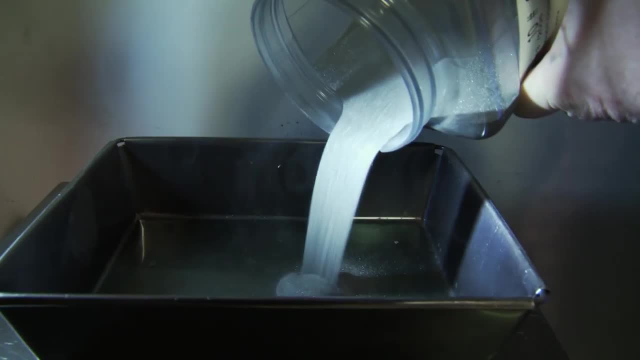 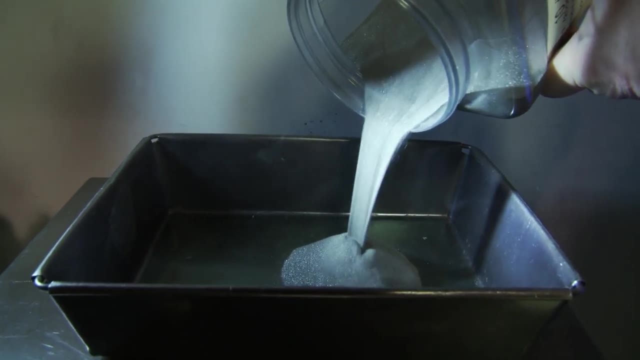 degrees celsius for many hours. In the sintering process, you basically, for a given material, you'll take powder that can react to a temperature, and that temperature has to be below the melting temperature, and so this process is different from a melt forging process: It's a densification. 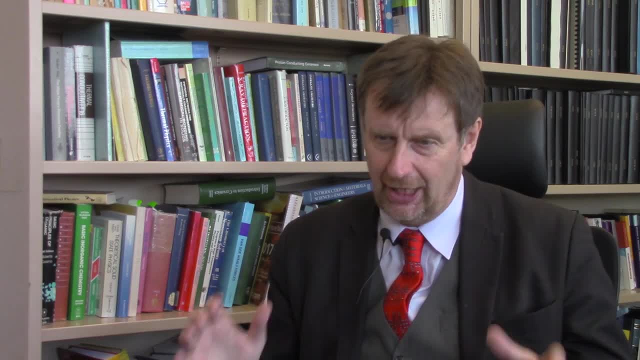 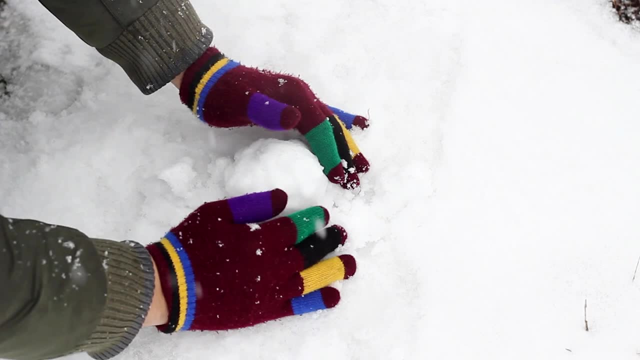 that is driven by molecules and atoms moving at the surfaces of these interfaces and minimizing that total amount of surface energy. Even the process, one could argue, of making a snowball is the compaction of particles and then applying some pressure with them. maybe there's a local 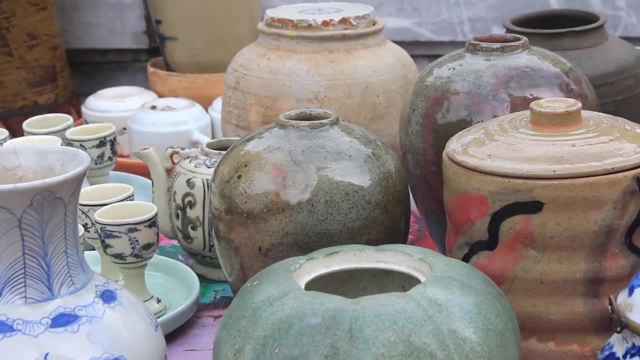 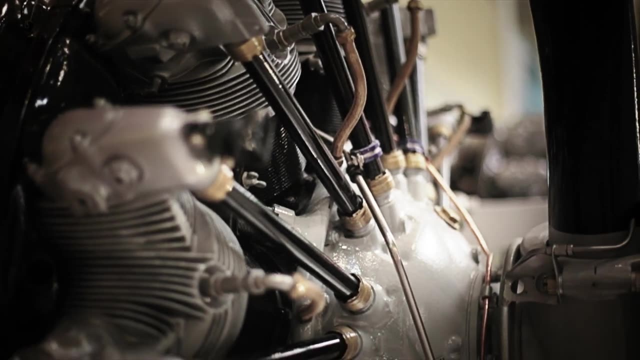 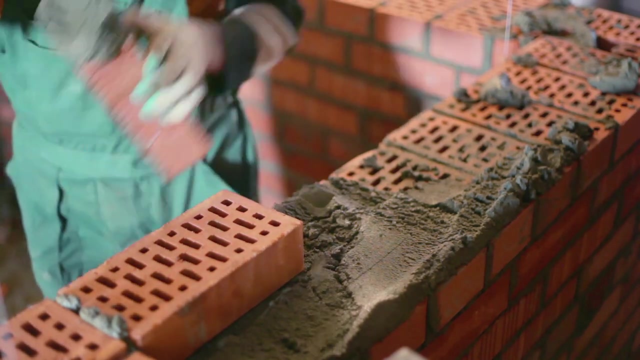 melting in the process. People have been sintering ceramics, metals, plastics and other materials for thousands of years. Today, sintering is used to create a wide variety of materials: Refractory materials used for brick technologies, tiles, alumina and zirconia bearing type materials. 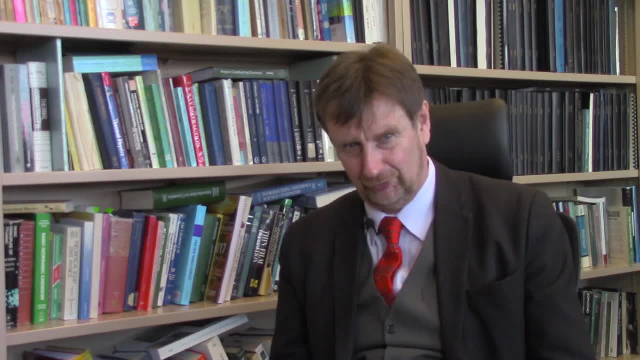 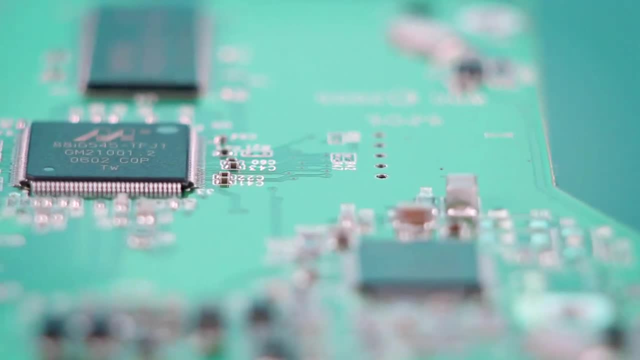 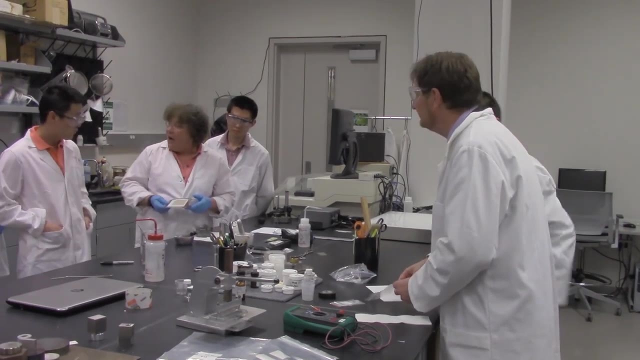 and pipes, very small functional materials for capacitor technologies. So, for example, in your iPhone you may have 700 pieces of ceramics and you may have 700 pieces of plastic ceramic all around capacitors. Three trillion of them are made per year. Randall and his team have developed a new technique where dense ceramics can be achieved.